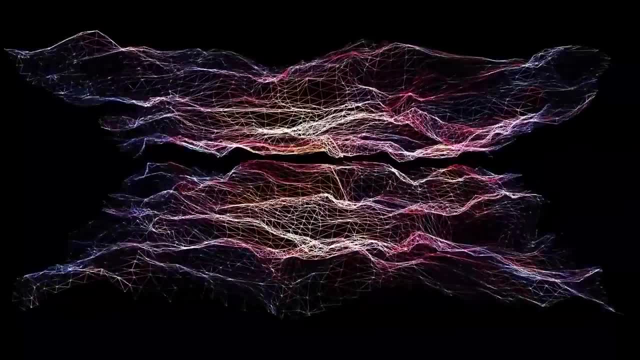 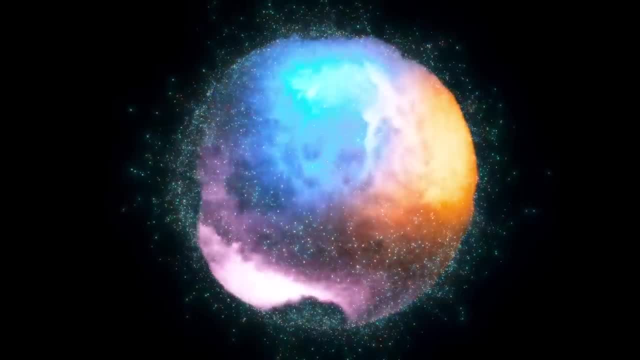 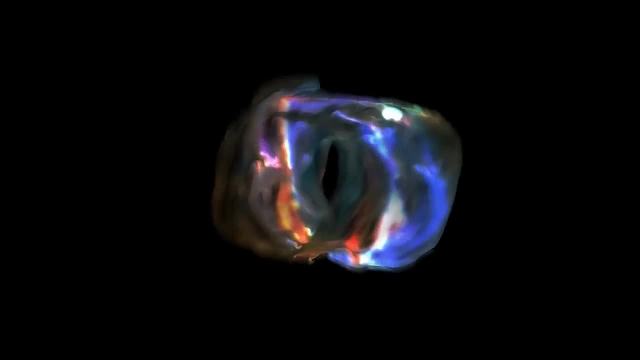 the universe. The universe is a symphony of strings. This is the mysterious world of quantum physics. As we explore the strange and fascinating phenomena of the subatomic world, where particles behave in ways that defy our everyday understanding of reality, we will oversimplify these concepts. 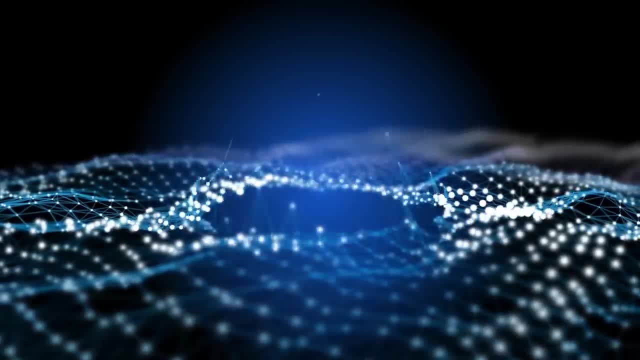 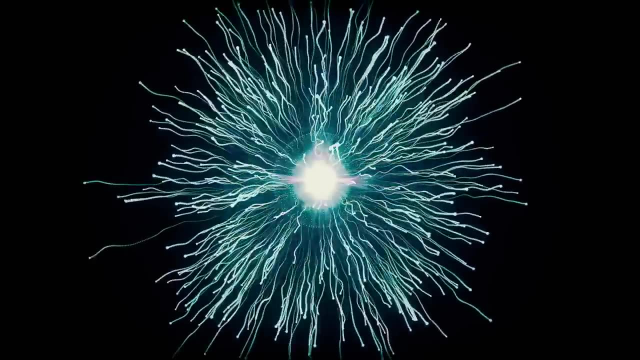 and hopefully you will forgive us for doing so, Because there is nothing harder to understand in science than quantum physics. As Richard Feynman once said, if you think you understand quantum mechanics, you don't understand quantum mechanics. At the heart of the quantum world lies the atom. 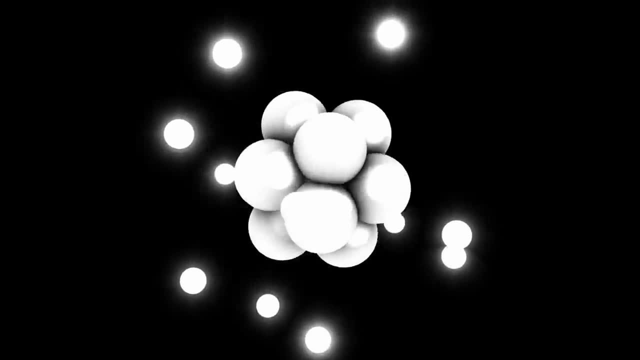 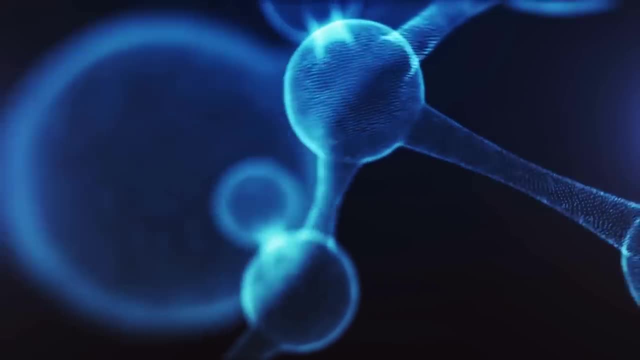 the building blocks of matter that were once thought to be indivisible. But as physicists delve deeper into the atomic world, they discover that the atom is not the only thing that is visible. They discover that particles don't behave like the everyday objects we encounter. 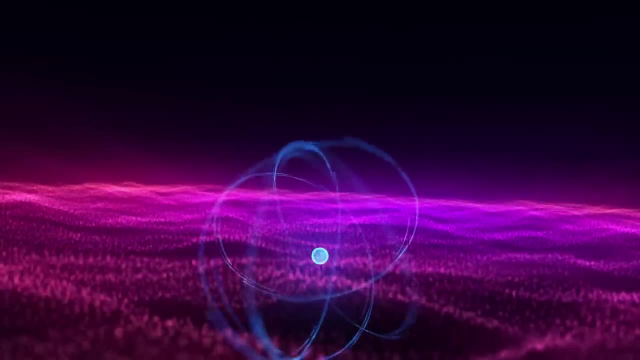 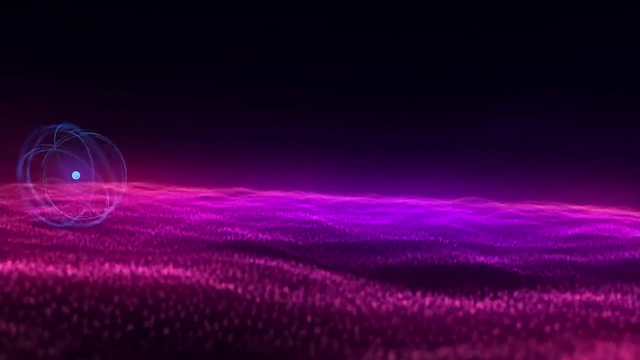 In the quantum world. particles exist in a cloud of probability. They can be in two places at once and have a mysterious connection that Einstein called spooky action at a distance. To make things even more bizarre, particles seem to be influenced by the observer as if they are aware. 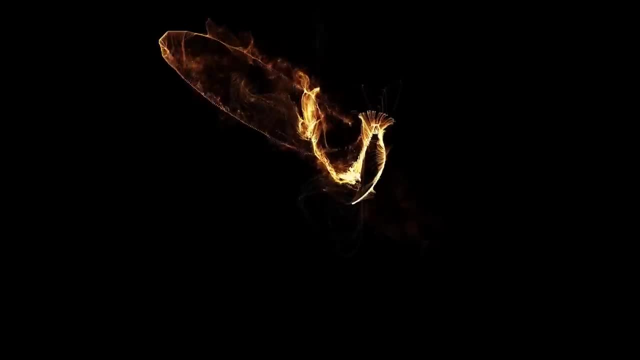 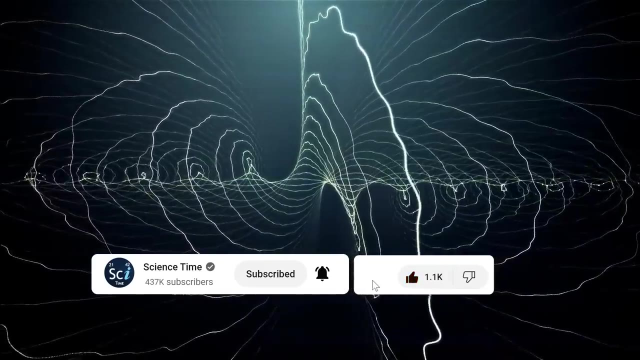 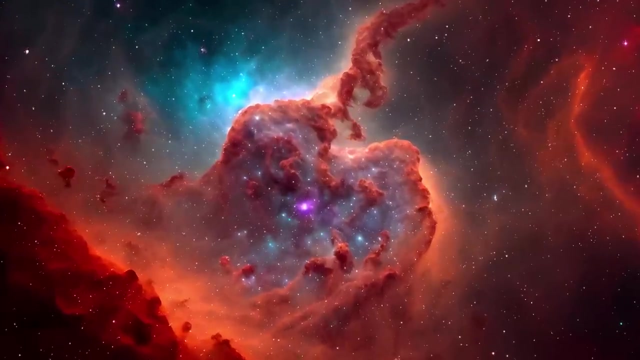 of being watched. But that's not all. String theory takes us even deeper into the mysterious world of subatomic particles. According to this theory, particles are not tiny dots, but tiny strings that vibrate at different frequencies, creating the variety of particles that make up our universe. It's fascinating to 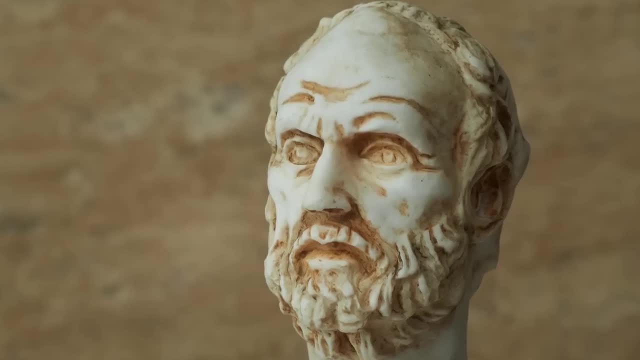 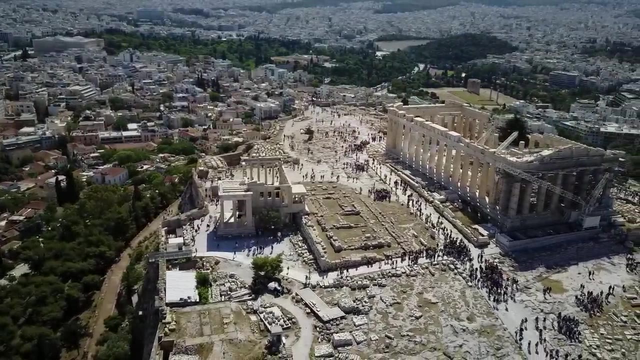 think that thousands of years ago, ancient Greek philosophers such as Democritus attempted to understand the atomic world using reason and logic. You know, Pythagoras was a rival of Democritus. Democritus talked about atoms 2,000 years ago. 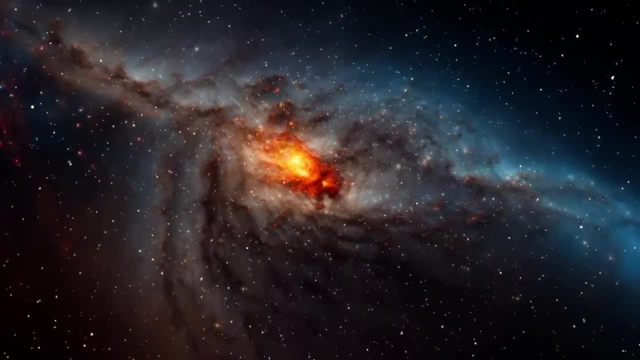 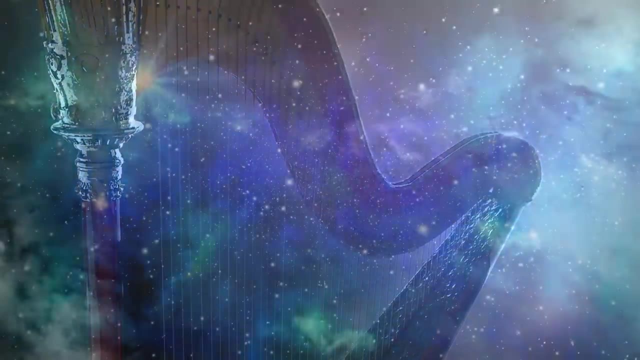 And Pythagoras said: no, no, no, Music is a language of the universe. So he looked at a lyre string and said: look at the vibrations. Each vibration corresponds to a musical note. The universe is music. The universe is created. 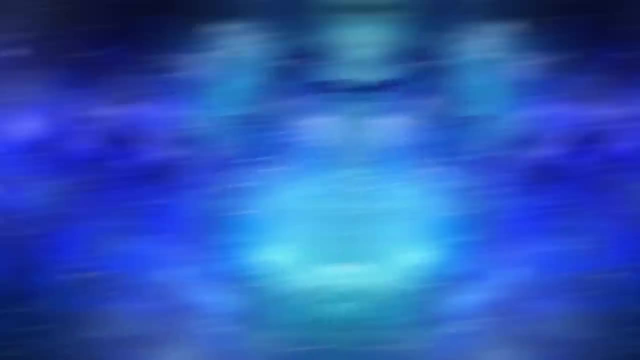 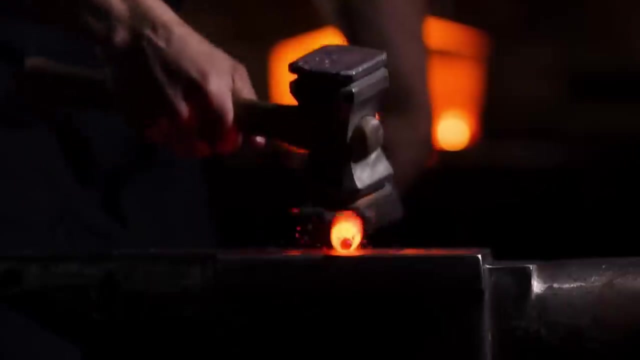 by vibrating things. Each vibration corresponds to a note. He went to a blacksmith where there were long bars of metal and they were clanging these bars of metal. He realized that the longer the metal, the lower the note. There's a relationship between the length of the object. 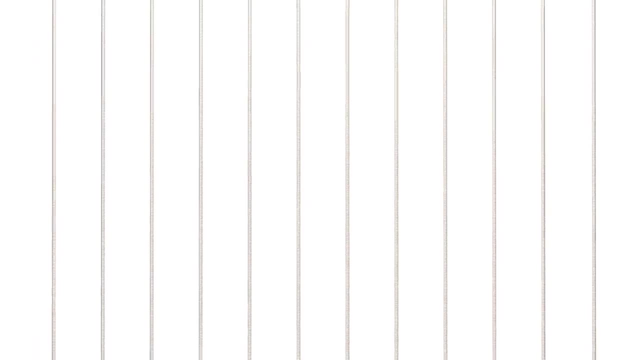 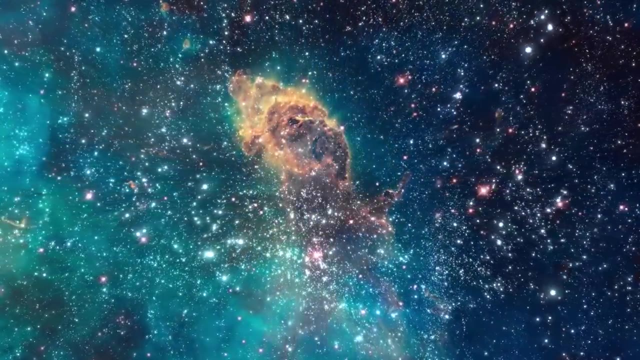 its strength and the note. And then he looked at a lyre string and he said: the longer the lyre string, the lower the note. And then he said: this is the universe. What explains the diversity? What paradigm is rich enough to explain the diversity of the entire? 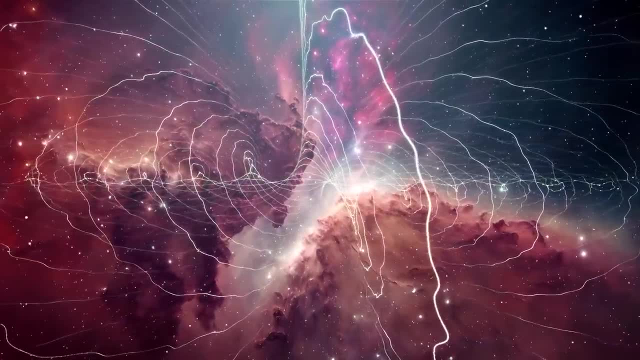 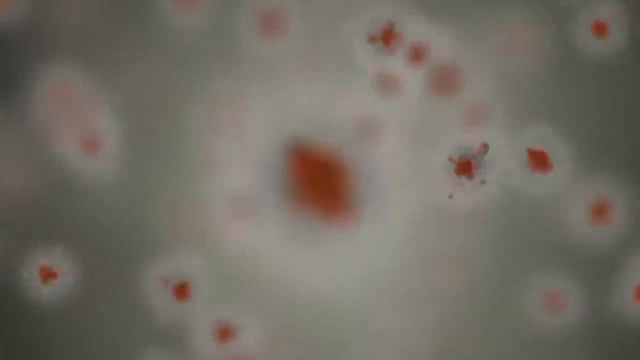 universe, Atoms. but what makes atoms different? And then he said it's music. But then that never went anywhere because of course the atomic theory wasn't created for another 2,000 years. But finally, with the atomic theory we now have subatomic particles. But why do we have so many? 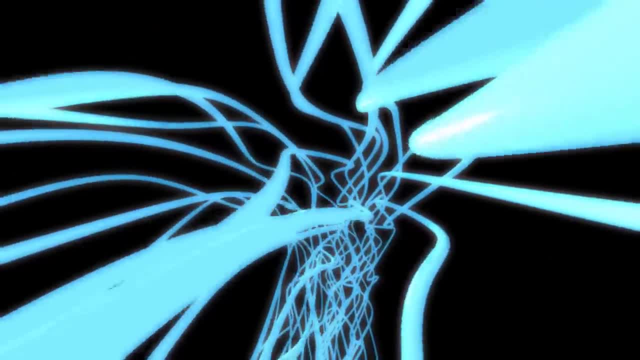 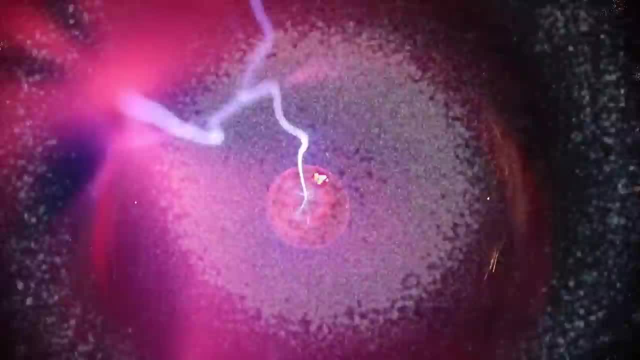 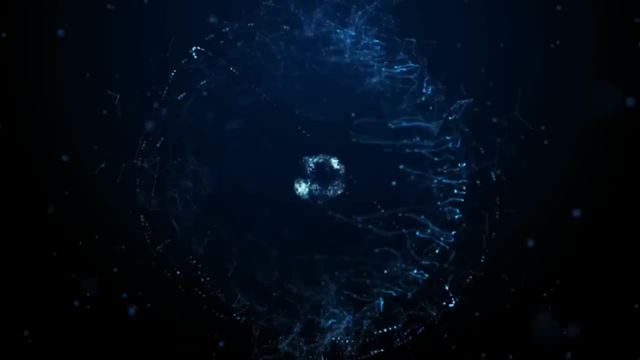 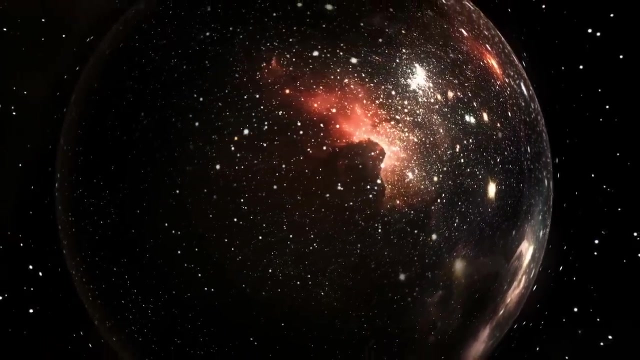 so many particles in the particle zoo. They're nothing but vibrations on a tiny string. String theory has also led to some intriguing ideas, such as the possibility of a multiverse where our universe is just one of many. While this idea is purely theoretical, it shows that the 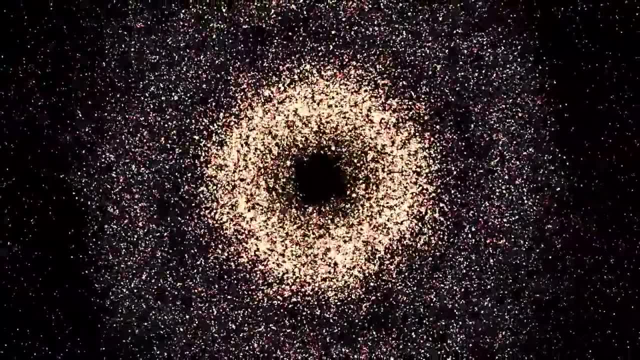 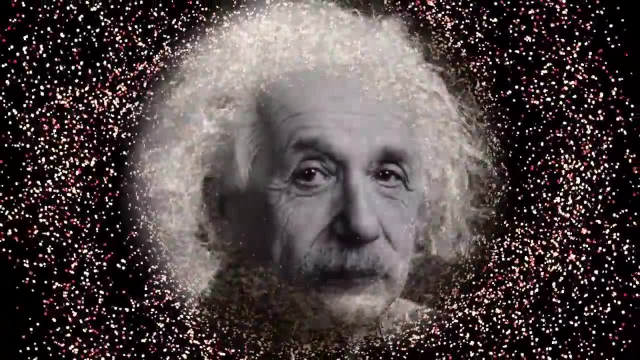 quest to understand the subatomic world is far from over. Some of the greatest minds in science have struggled to understand quantum theory. One of the most notable was Albert Einstein, who believed in a hidden reality that we can't directly observe. He rejected the idea of 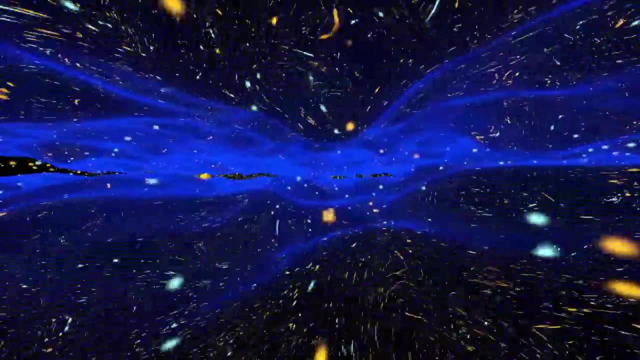 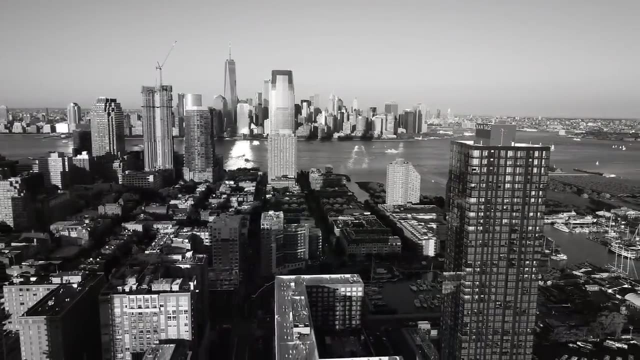 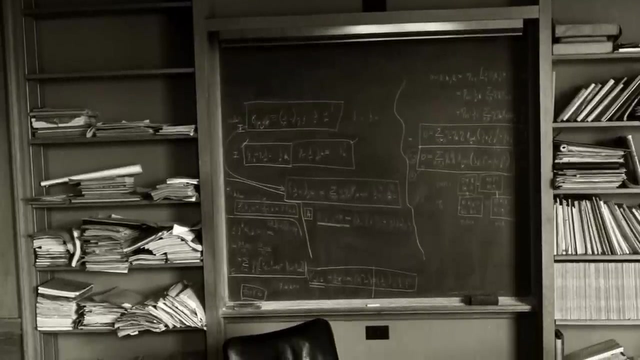 entanglement. but as experiments continued to prove the validity of quantum theory, Einstein's views became increasingly marginalized. When I was eight, something happened to me as well: It was in all the papers that a great scientist had just died, and they put a picture of his desk on the front page. 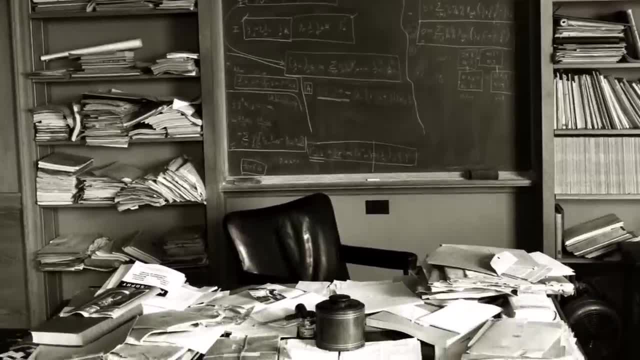 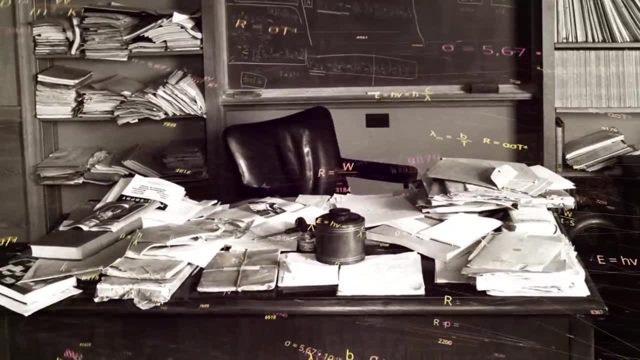 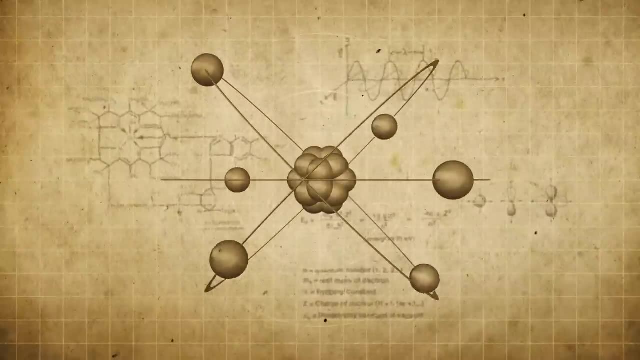 That's it just a simple picture of the front page of the newspapers of his desk. That desk had a book on it, which was opened and the caption said more or less: this is the unfinished manuscript from the greatest scientists of our time. So I said to myself: well, why couldn't he finish it? 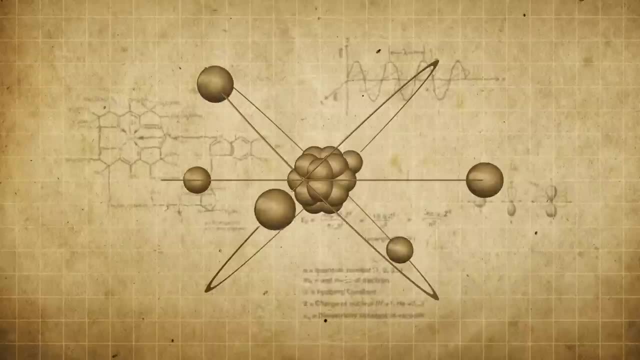 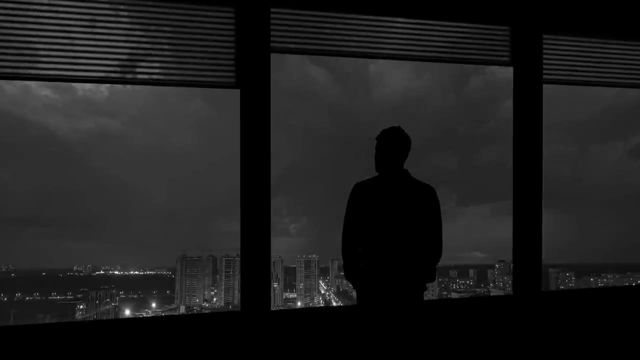 What's so hard that you can't finish it. if you're a great scientist, It's a homework problem, right? Why couldn't he solve it? So to me, this was a murder mystery. This was greater than any adventure story. I had to know why the greatest scientists of our time 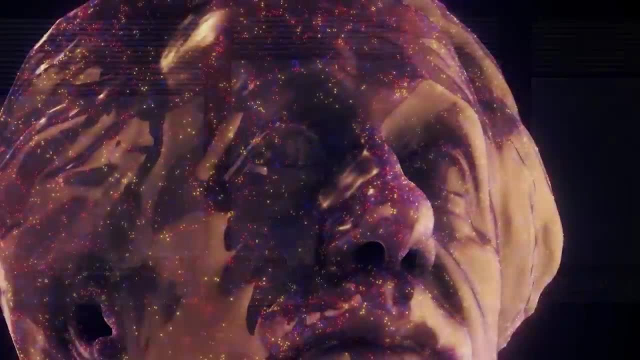 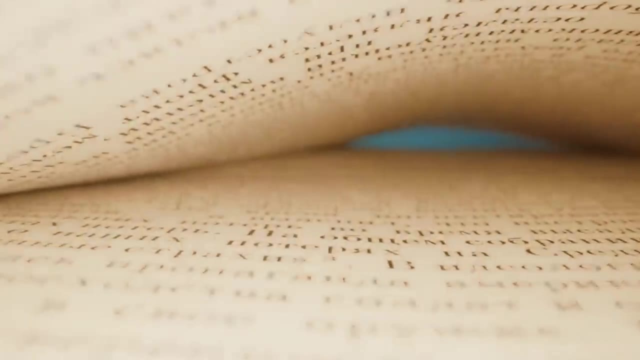 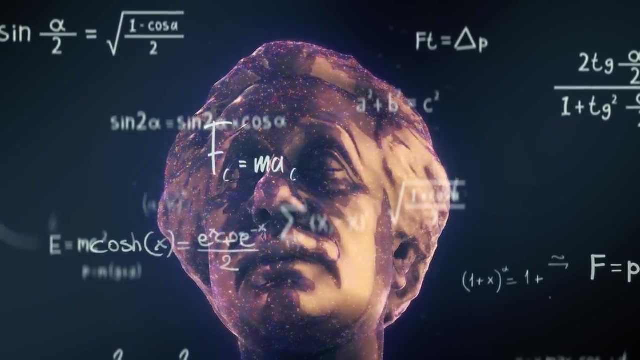 couldn't finish something. And then, over the years, I found out the guy had a name, Albert Einstein, and that book was the theory of everything. It was unfinished. Well, today I can read that book, I can see all the dead ends and false starts that he made and I began to realize. 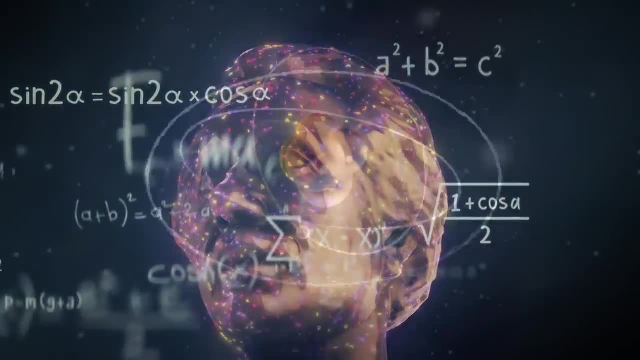 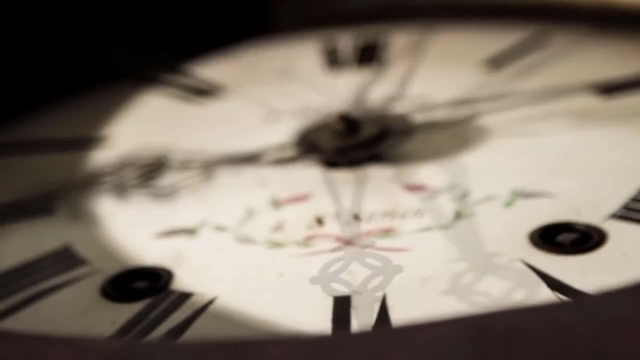 that he lost his way. I can see all the dead ends and false starts that he made and I began to realize that he lost his way Because he didn't have a physical picture to guide him on the third try. On the first try he talked about clocks and lightning bolts and meter sticks and that gave us. 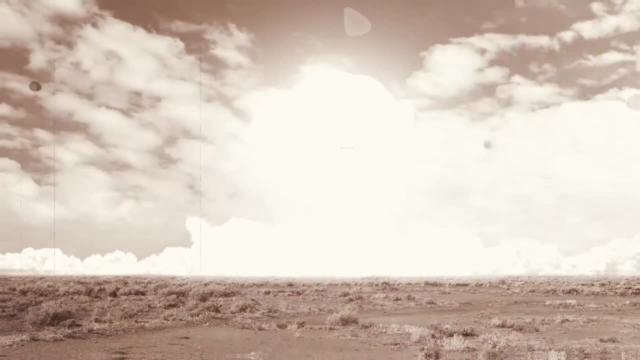 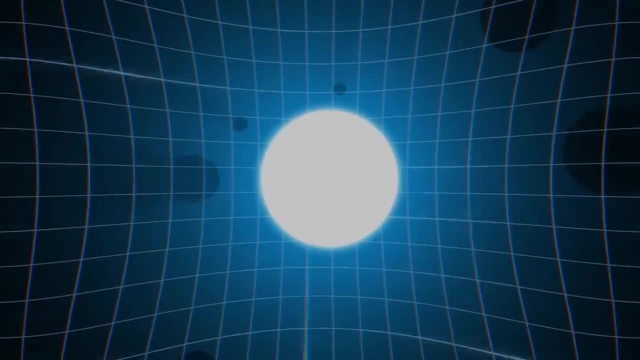 special relativity, which gave us the atomic bomb. The second great picture was gravity, with balls rolling on curved surfaces, and that gave us the Big Bang, creation of the universe, black holes. On the third try, he gave us the atomic bomb. and that gave us the atomic bomb, The second. 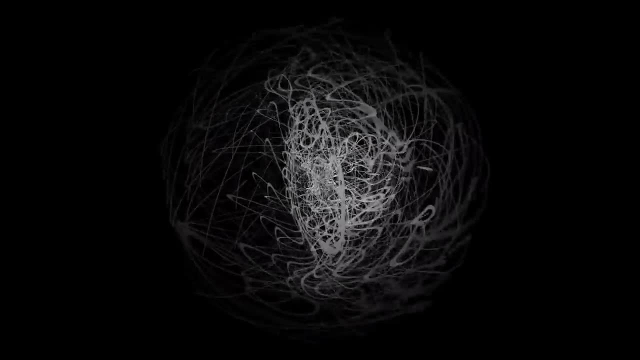 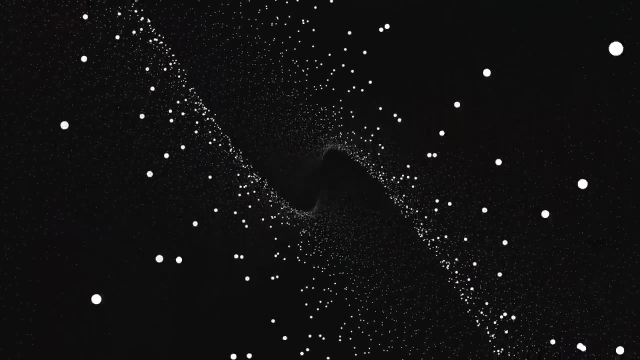 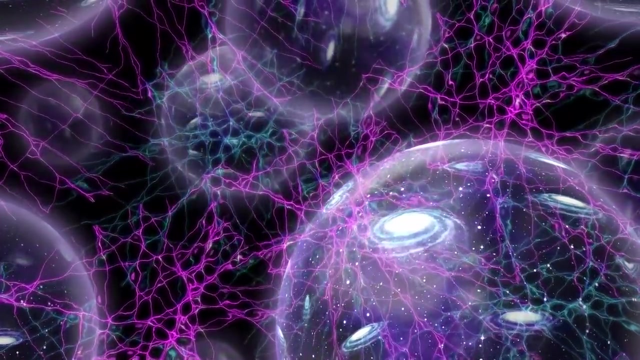 he missed it. He had no picture at all to guide him. Well, today we think that picture is string theory. String theory also proposes the existence of extra dimensions beyond the three we are familiar with. It's a mind-bending concept that raises the possibility of multiple universes. 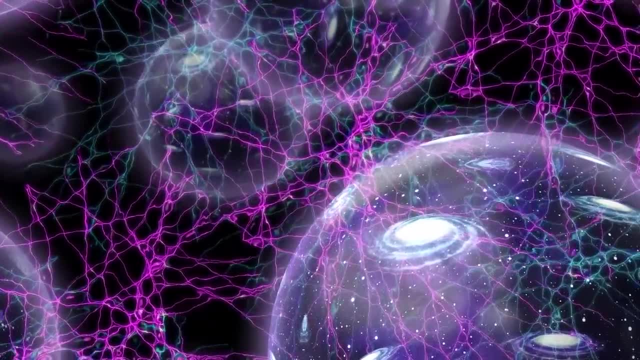 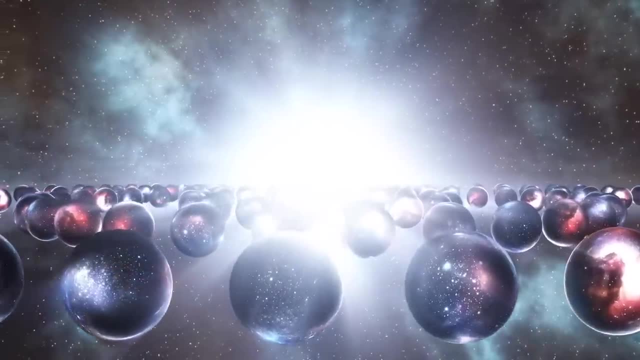 each with their own set of physical laws. These parallel universes, also known as the multiverse, are a popular topic in science fiction, but they are also a serious area of study for scientists. The idea is that every time there is a decision to be made, the universe 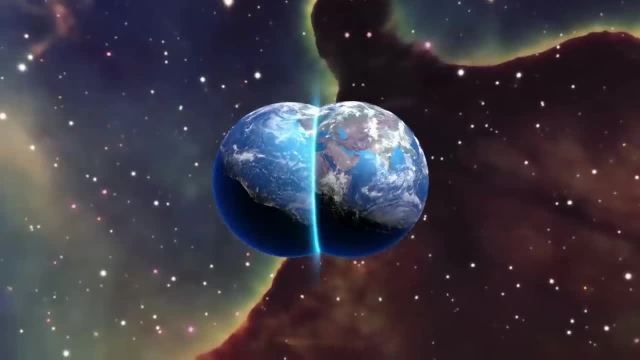 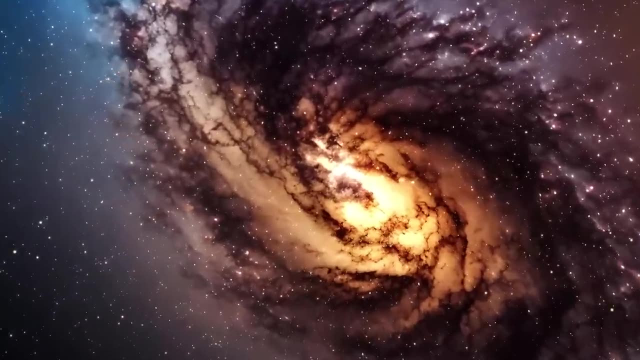 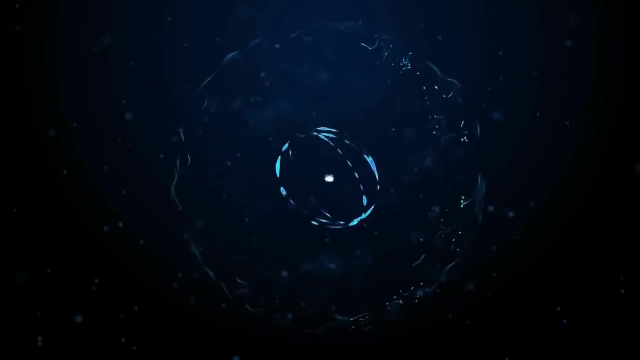 splits off in two or more possible outcomes, each occurring within its own separate universe. String theory could also help explain the mystery of dark matter. This mysterious substance makes up around 27% of the universe, but we can't directly observe it. One explanation is that 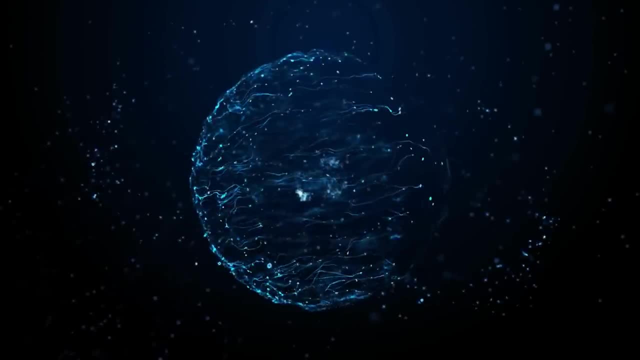 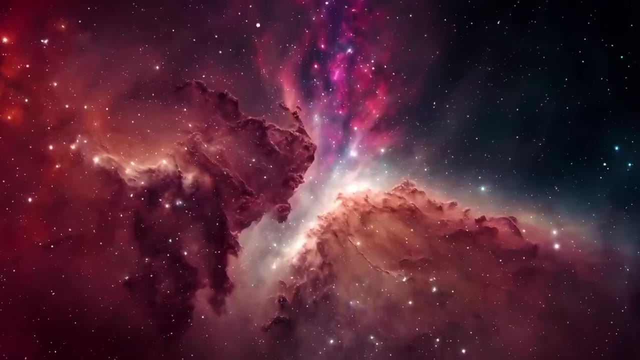 dark matter is made up of particles known as WIMPs, Weakly Interacting Massive Particles which could be used to measure the size of the universe. The WIMPs are made up of particles produced by the vibrations of strings. While there is still so much we don't know about string. 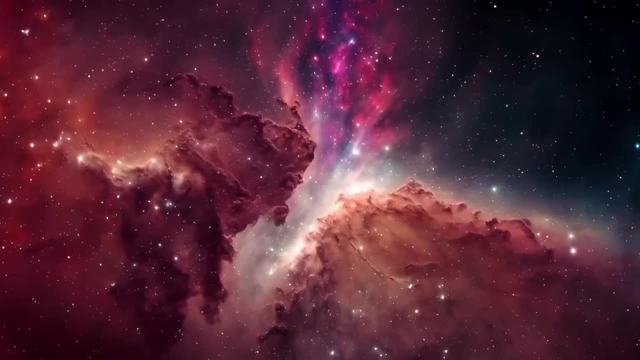 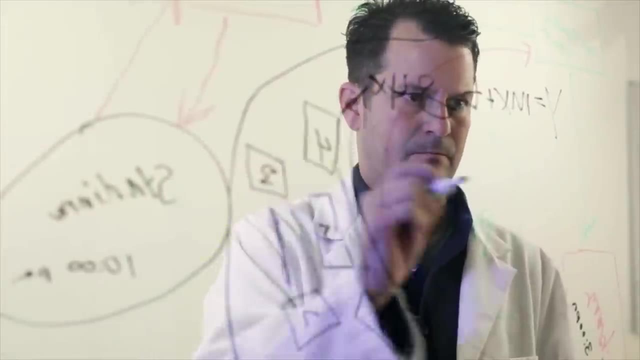 theory. it has opened up new avenues of research and shown us that the universe is far more complex and wondrous than we ever imagined. However, string theory or, to be more accurate, the string hypothesis, has also been heavily criticized by the scientific community.